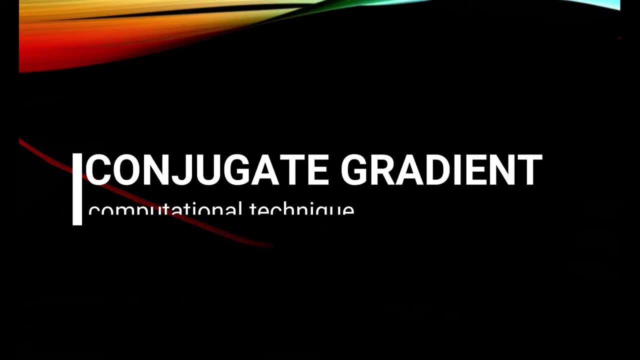 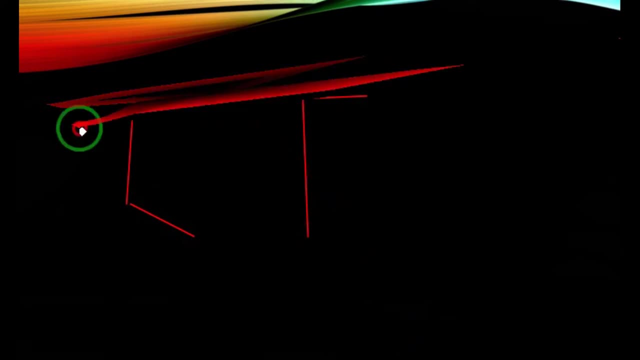 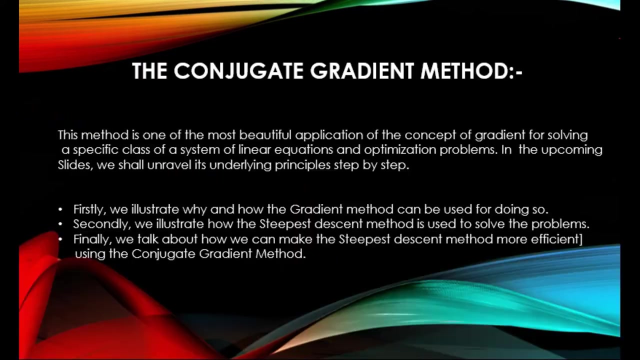 Hello, Namaste, and welcome to this video series where we'll be focusing on the various underlying concepts of different methods used under the computational technique and demonstrate their applications by practicing some numerical problems. But today we will be looking at the conjugate gradient method. Well, the conjugate gradient method is one of the iterative methods. 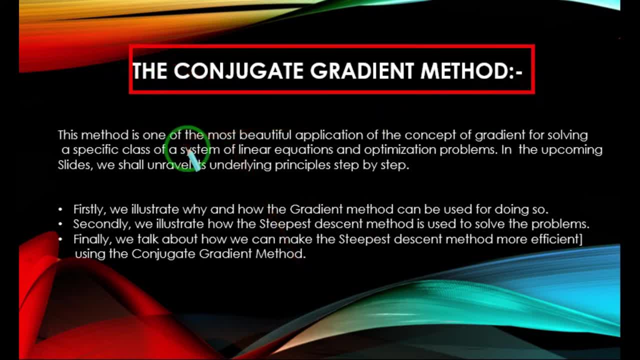 with a high rate of convergence, which basically means that this method converges or approaches the solution at a faster rate, which again means using a fewer number of steps. Well, this method is one of the most beautiful applications of the concept of gradient for solving a specific. 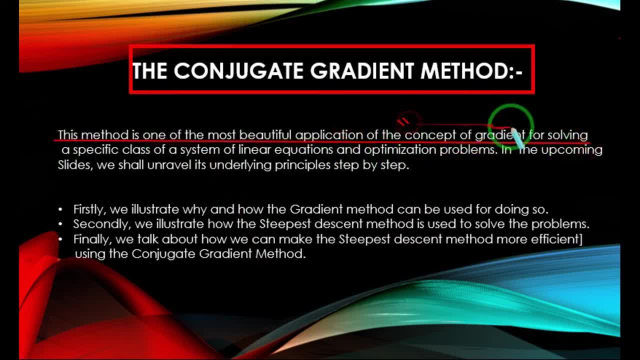 class of a system of linear equations and optimization problems. In this video we shall explain its underlying principles One step at a time. Firstly, we will illustrate why and how the gradient method can be used. Secondly, we will illustrate how the steepest descent method is used to solve the problems. 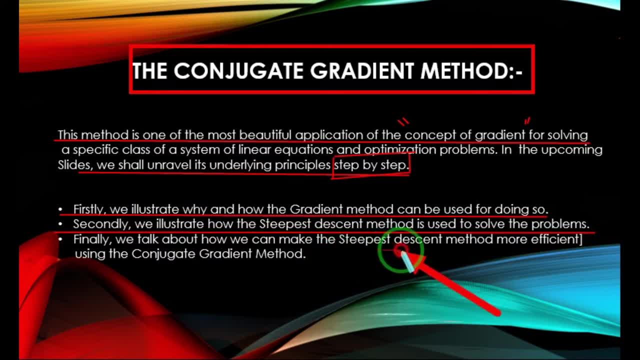 And finally, we will talk about how we can make the steepest descent method more efficient by using the conjugate gradient method. Well, time to pause and reflect a bit. Before proceeding further in digging into this method, make sure that you subscribe to our channel, and. 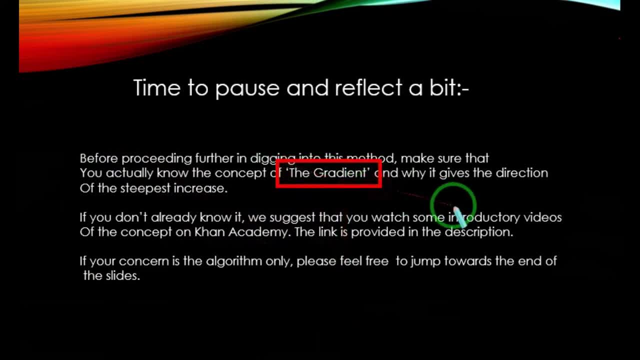 that you actually know the concept of the gradient and why it gives the direction of the steepest increase. Well, if you don't already know it, we suggest that you watch some introductory videos of the concept on Khan Academy. Well, the links are provided. 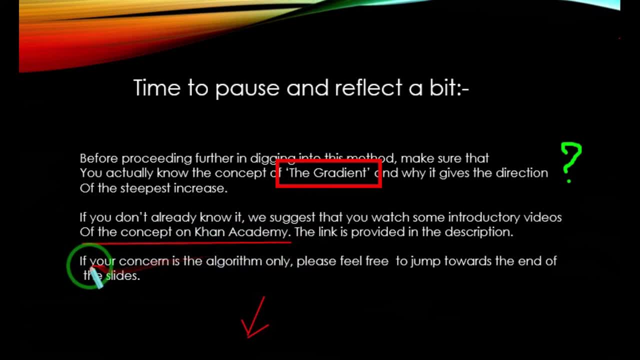 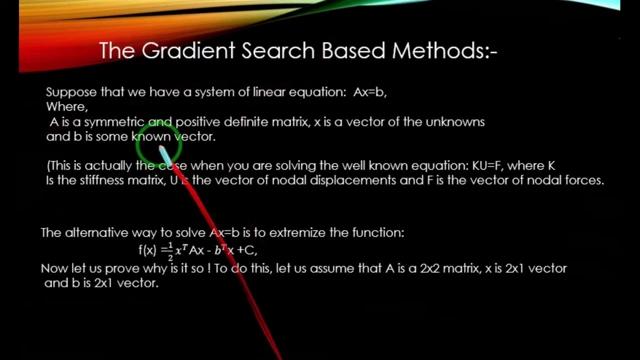 in the description. Do check them out. But if your concern is the algorithm only, please feel free to jump straight towards the end of the video. Now, without any further delay, Let's jump into the topic. Okay now, suppose that you have a system of linear equation which is given by the equation: 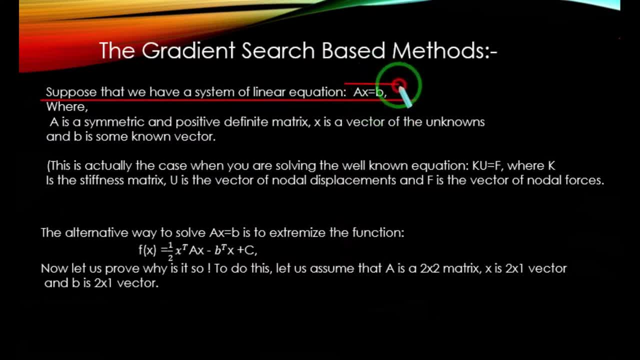 AX is equals to B, where A is a symmetric and positive definitive matrix, X is a vector of the unknowns and B is some known vector. Well, this is actually the case when you are solving the well-known equation K times U is equals to F, where 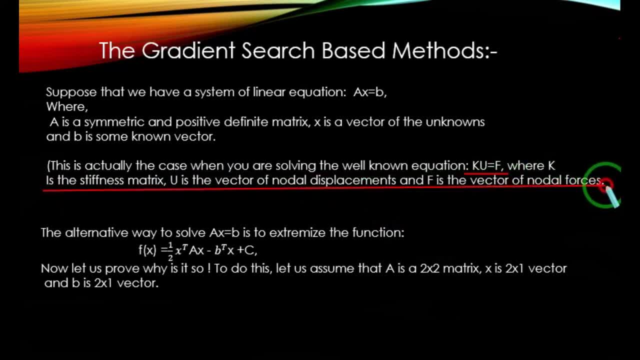 K is the stiffness matrix, U is the vector of nodal displacements and F is the vector of nodal forces. Well, that is basically the stiffness equation. Well, solving the linear equation AX is equals to B is equivalent to finding the minimum. 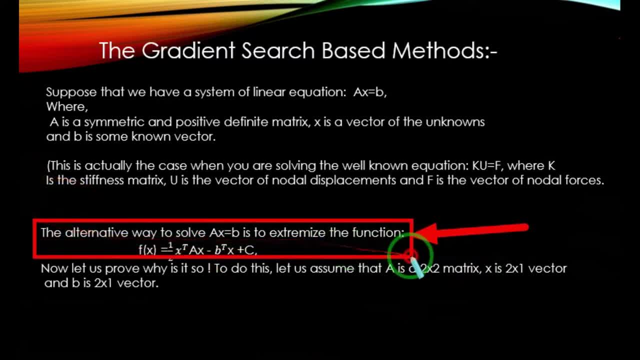 of the quadratic form. F is equals to half of X. transpose times A, times X minus B. transpose times X plus C, and its derivative is: its gradient is given by f. dash of x is equals to ax minus, and finding the minimum of f of x. 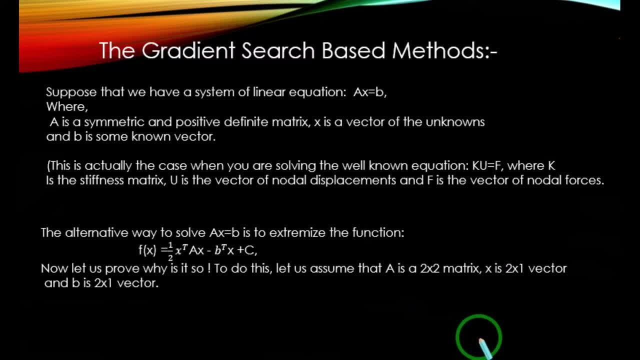 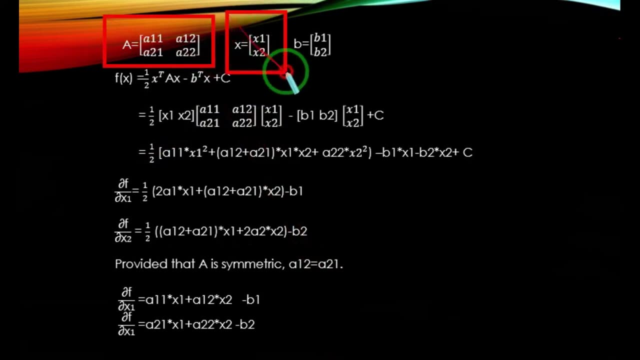 is the key to solving the system of linear equation: ax is equals to b. well, now let us prove why it is so, and to do this, let us assume that a is a two by two matrix, x is a two by one vector and b is a two by one vector as well. now, substituting these values of a, x and b. 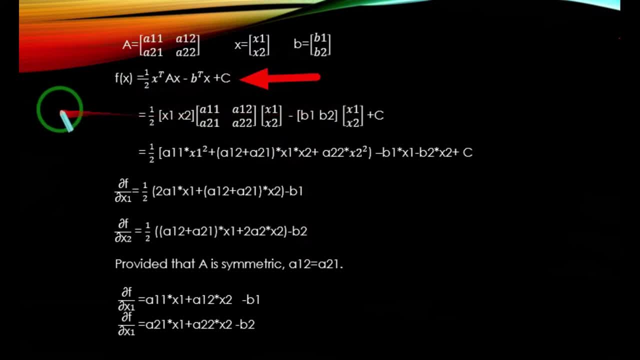 in the previously mentioned equation, f of x is equals to half of x. transpose times a times x minus b, transpose times x plus c, we get the following results: after a few steps of matrix multiplication, you finally get this equation. now, what is extremisation? well, we mentioned earlier. that if we run a three factor equation and we can actually add them to the f dash in a three to x value, well, first we are going to take a very specific medida and this is what we are going to recover. so now, if we run a three factor equation and we are going to drive down the lower milk number four- and this is what we are going to recover- 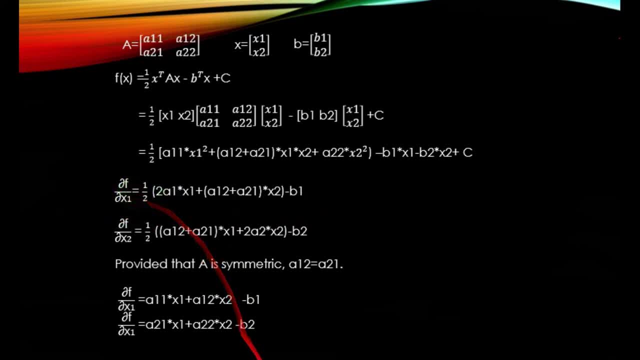 was simply finding the gradient of a function. well, in order to find the gradient of our given function, f of x, we simply differentiate it with respect to the unknown variables. now, taking x1 first. differentiating f with respect to x1, we get the following equation: similarly differentiating f, 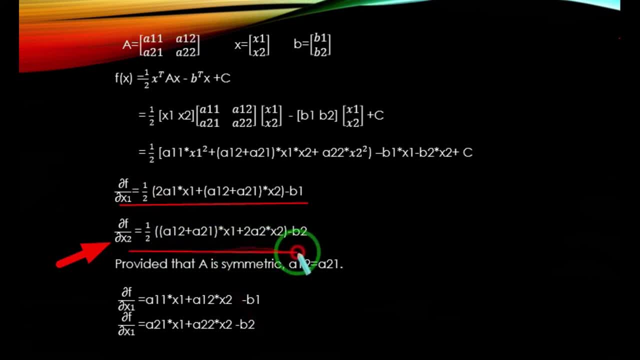 with respect to x2, we get the following output: now, provided that a is a symmetric matrix, a12 is equals to a21. well, that is simply: aij is equals to a ji. now, using this condition in the previously found equations, we get the following output: simply substituting a12 by a21, we get the following: 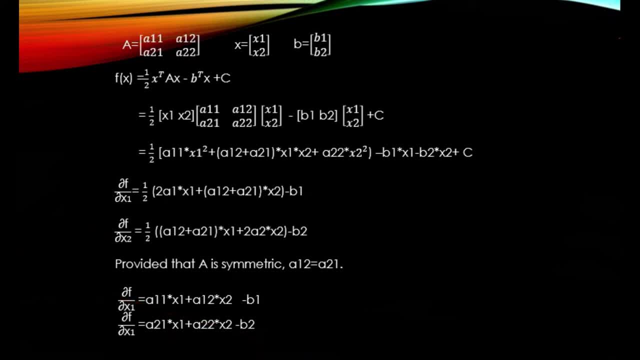 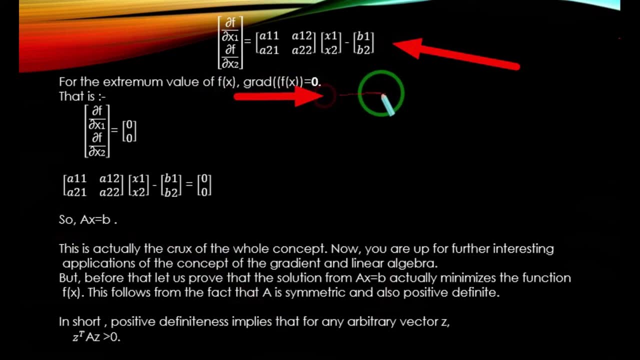 well, hope you guys are following us. well, what to do next for the extreme values of f of x? well, the gradient of f of x should be equals to, yeah, zero. well, since we are dealing with vectors and matrix, we will have to equate the gradient of f of x with the null vector as shown in the screen. well, the bold zero that. 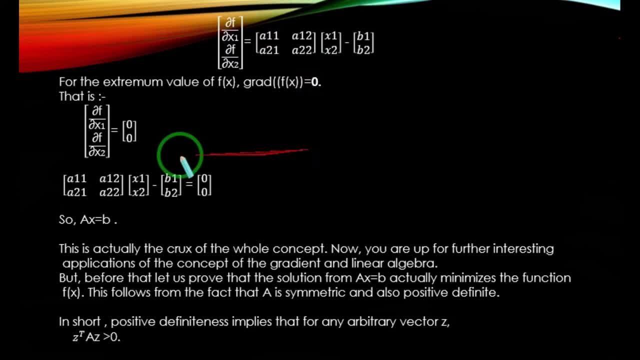 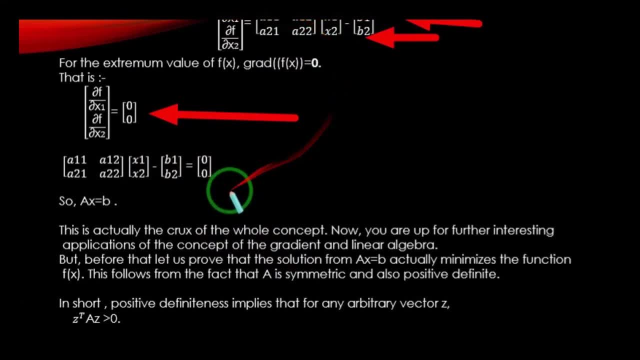 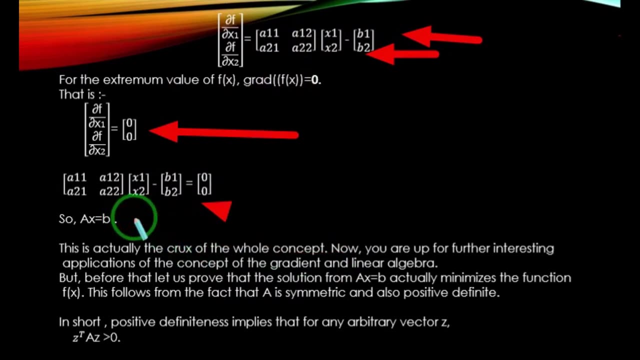 you're seeing is basically null vector. now, equating with the null vector and substituting the values, we simply get function no, ds, f of x. so actually's the correct of the whole concept. now you are up for further interesting applications of the concept of gradient and linear algebra, but beforeи that, let us prove that the resolution from ax equals to b actually minimizes the function of f of x. this can be written as an a times x equals b, which proves that our previously mentioned extremization function works well. this is actually the correct of the whole concept. now you are up for further interesting applications of the concept of gradient and linear algebra, but before that, let us prove that the solution from an x is equals to b actually minimizes the function of an. 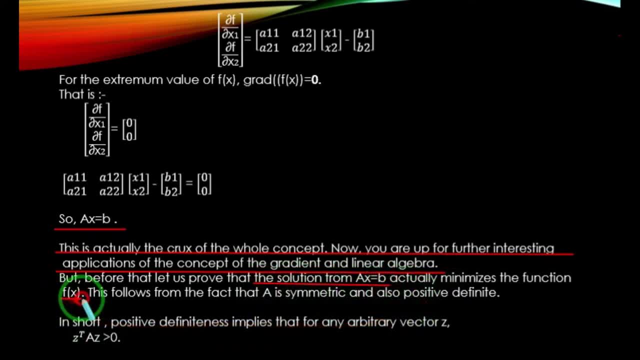 a equals to b actually minimizes the function f of x. well, this follows from the fact that a is a symmetric and also positive definitive matrix. well, in short, the positive definitiveness implies that for any arbitrary vector z, z transpose times a, matrix times. the vector z again should always. 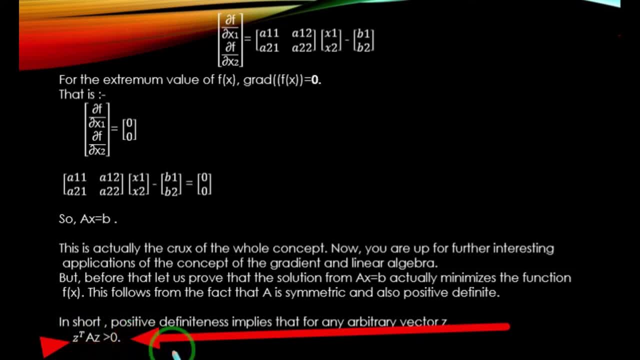 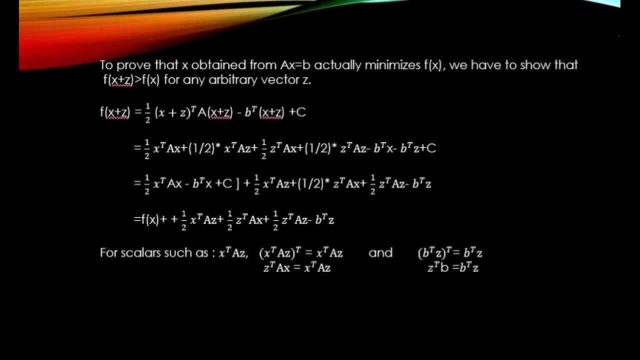 be greater than zero. well, the value. if it's positive, then the matrix a is a positive, definitive matrix. now, to prove that x obtained from ax is equals to b actually minimizes f of x. we have to show that f of x plus z is greater than f of x for any arbitrary vector, z. 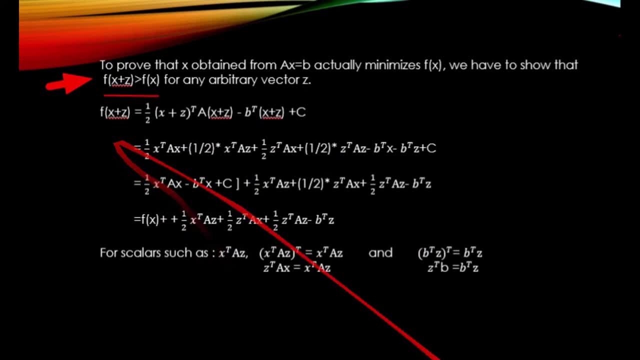 so? so what do we do? well, using the previously used extremization function and substitute x plus z instead of just x, we get the following output: after a series of steps, now now. now, now for scalars such as x, transpose times a times z, you can see this form of equation: 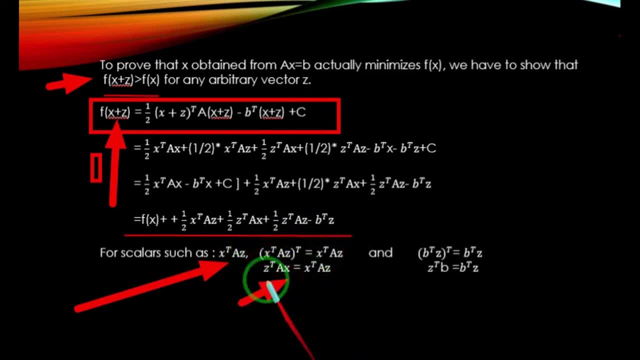 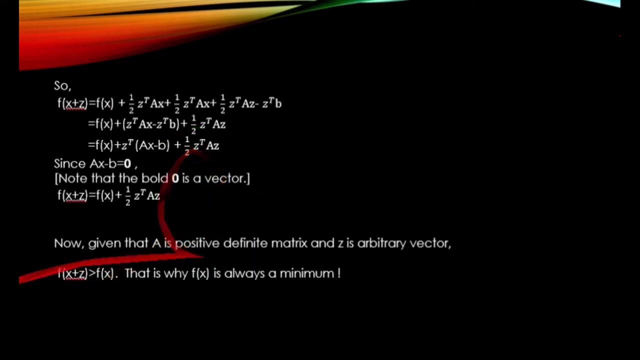 is derivable, right, is it okay? well, this can be obtained, because a is a symmetric matrix and simply using the property of transposition, we get these outputs. now, substituting the these outputs in the previous equation, you get something like this: hope you guys are following now, since a, x minus b is equal to a null vector. well, note that the bold zero you're seeing there. 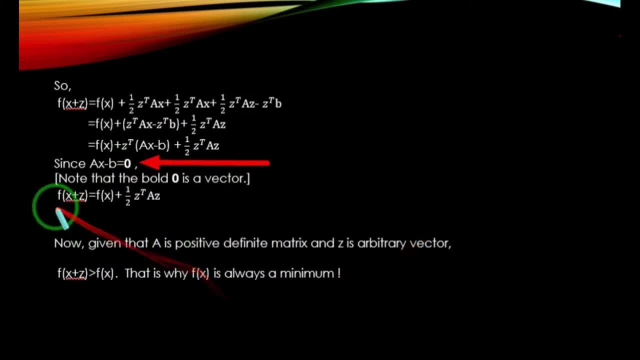 is a vector. so this gives us f of x plus z is equals to f of x plus plus something, guys, plus something plus half of z. transpose times a. x. transpose times a. x. transpose times a. x. transpose times a times z. now, since a is a positive, definitive matrix, this expression of half of z 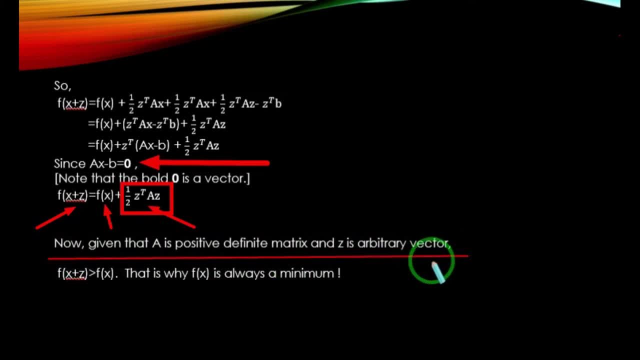 transpose times a times. z is always positive, which clearly implies that f of x plus z is greater than f of x. that is why f of x is always a minimum. now moving into the steepest descent method, we know that the gradient of f of x at a point gives: 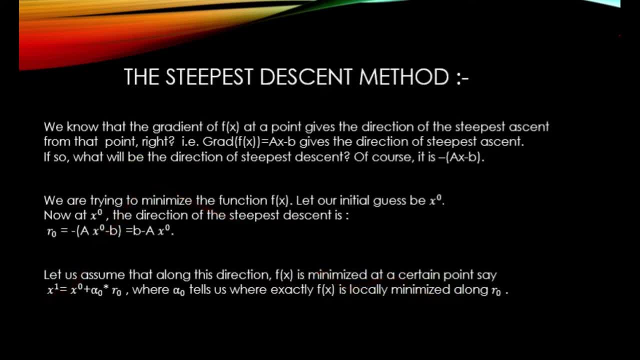 the direction of the steepest ascent from that point right? well, that is. gradient of f of x is equals to a x minus b, which gives the direction of the steepest ascent. if so, what will be the direction of the steepest descent? well, of course it is negative of a x minus b. we are trying to 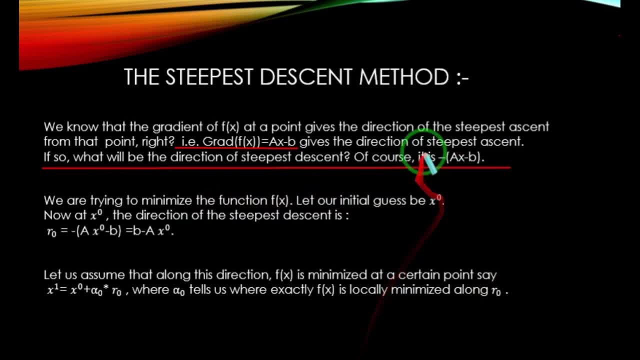 minimize the function f of x. so let our initial guess be x naught, x zero, whatever you call that. well now, at x naught, the direction of the steepest descent is given by r naught, which is equals to negative of a x naught minus b, which can simply be written as b minus a times x naught. now let us 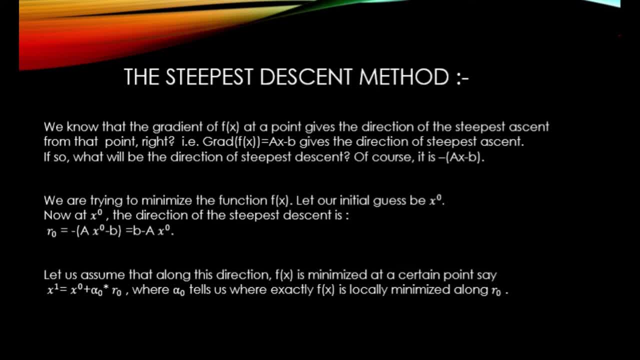 assume that along this direction f of x is minimized for a certain point. say x 1, which is equals to x naught plus alpha naught times r naught. well here alpha naught tells us where exactly f of x is locally minimized. along r well with that, simply. 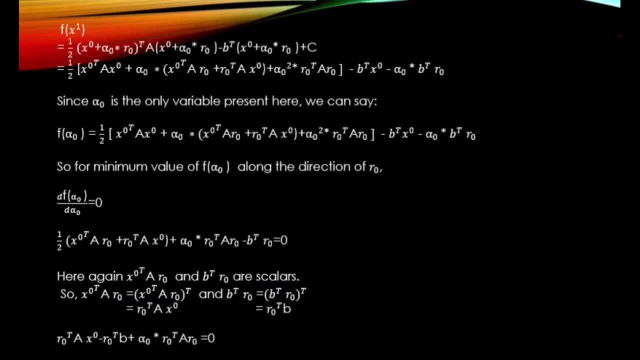 using the following outputs: using the following obtained conditions in the extremization function with f of x 1, you get the following output: simply substituting the values, you get something like this: well now, since alpha naught is the only variable present there, we can say: f of alpha naught is equal to half of x naught. transpose times a times x naught plus alpha naught. 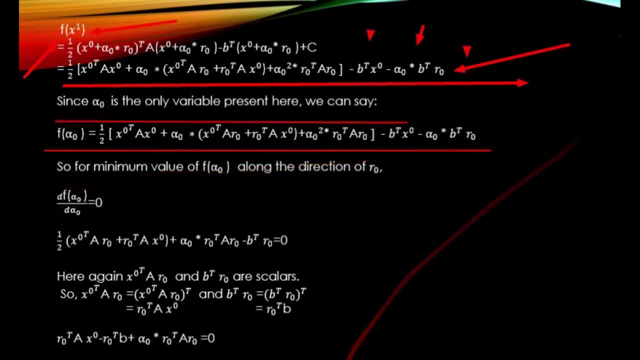 times. oh, my god, guys, you can just clearly see that right. well, after a series of steps, you simply obtain these, you can simply obtain this form. so well, let's continue so. for minimum value of f of alpha naught along the direction of r naught, which is given by derivative of. 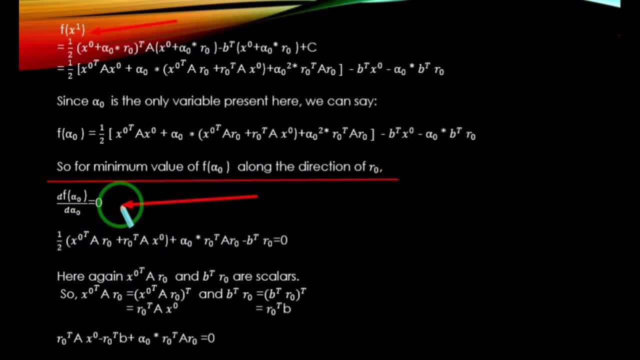 f of alpha naught with respect to alpha naught, which we equate with zero. now, equating with zero, using the above obtained equation and equating with zero, you get something like this. now, here again: x- naught transpose times a times r naught and b transpose times r naught, r scalars. so so so. 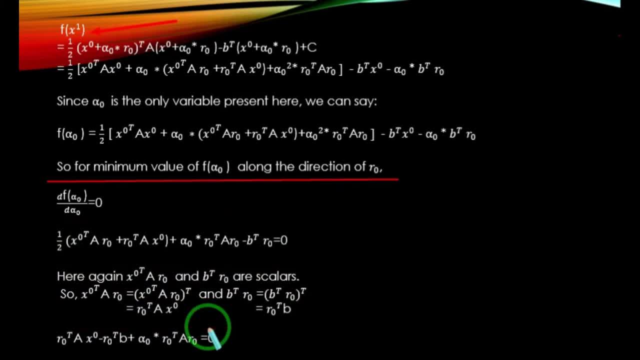 x naught. transpose times a times r naught is equals to r naught. transpose times a times x, naught and b. transpose r naught is equals to r naught. transpose times b. right, yes, guys, if you're having a hard time following me, you can just simply write down the steps and copy and that'll. 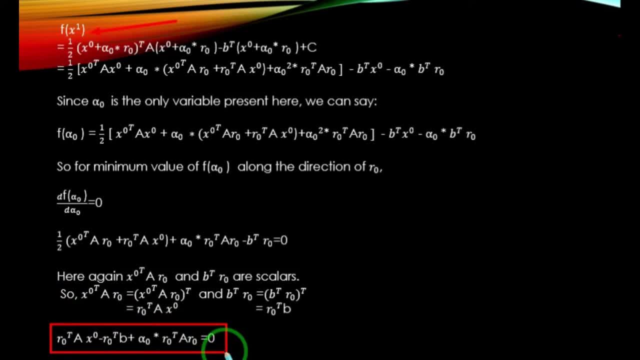 be clear. that'll be more clear and easy to understand. well, uh, computational techniques consist of a lot of mathematical writing, so it's a little hard to grasp simply looking at this. well, after a series of steps- again guys- you obtain this form of equation, now substituting: 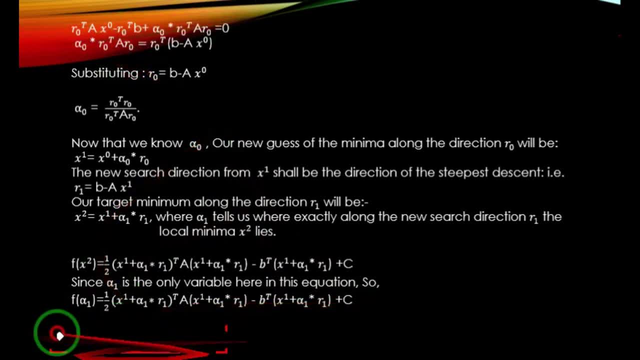 r naught is equals to b minus a times x naught, you get alpha. naught is equals to r naught transpose times r naught divided by r naught. transpose times a times r naught. well, it's important that you shouldn't simply write that down, because you will get that anyway. 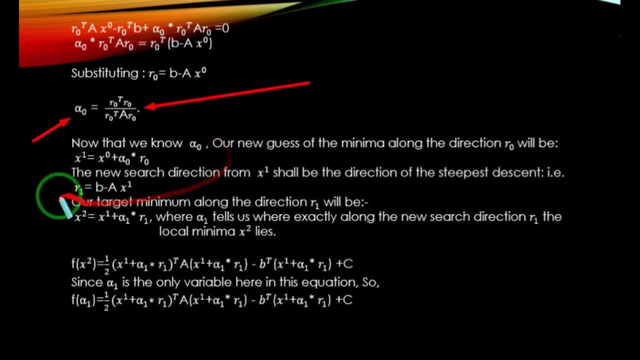 now we just need to describe that with the first phase of Princess right here, which is: d is equal to one after and d is equal to minus b, because minus is one and d equals b plus, so that's one and b minus is equal to one. just let's say: you here have to bring some shape right here, like we did in the first step. 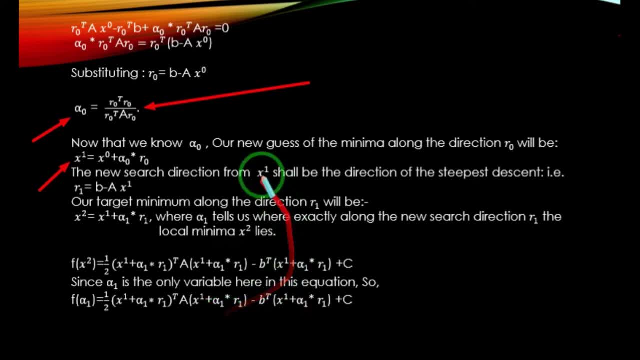 so let's first bring in your first two derivatives now, as we said before, from the pipette section. then from the other side, you might use thetycznie interval. you would to combine both as you like. you've done this right. so here's where you're going to end up. we're going to cross the situation here. 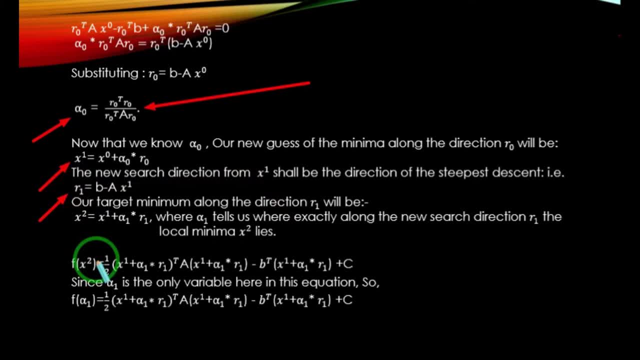 the direction r1 will be. x2 is equals to x1 plus alpha 1 times r1. guys, we are simply repeating the same process. well, this is an iterative method, so you'll be simply repeating again, and again, and again till you converge to the point with 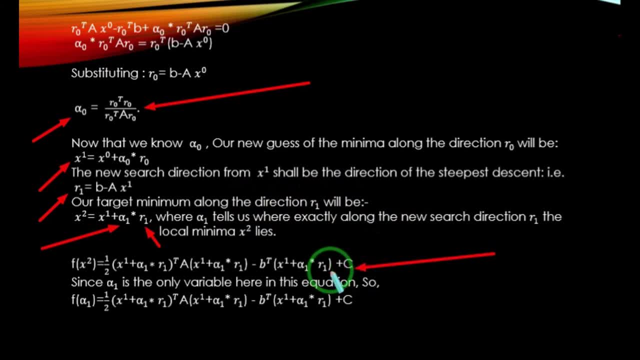 permissible tolerance. well, here, r1 tells us where exactly along the new search direction. r1, the local minima x2, nice. well again, using the extremization function on x2, f of x2 is equals to half of x1 plus alpha 1 times r1 transpose. 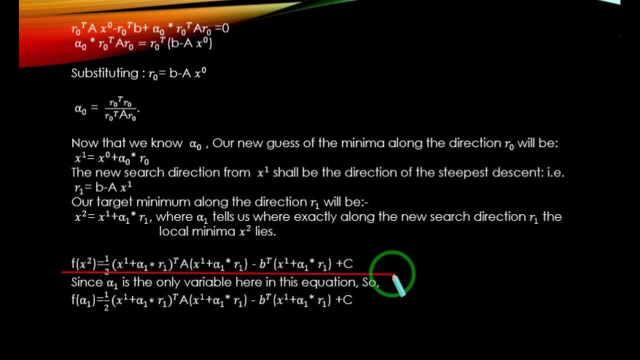 times a times x1 plus alpha 1 times r1 minus B. transpose times x1 plus alpha 1 times r1 plus C. well, since alpha 1 is the only variable here in this equation, we can use the same method to find the value of alpha 1 times r1 and. 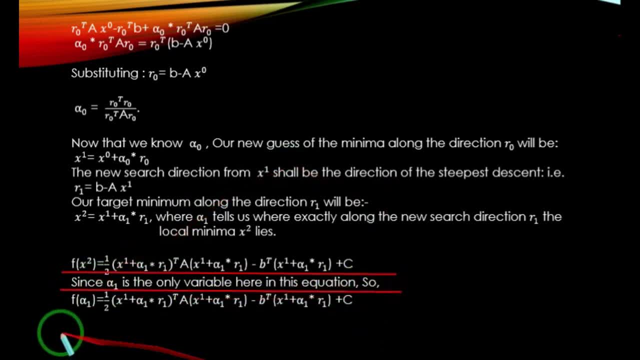 we can use the same method to find the value of alpha 1 times r1 and we can use this equation, so finding half of alpha one. you'll get something like: clearly see on the screen. guys can practice it down in your copy and you will just this: 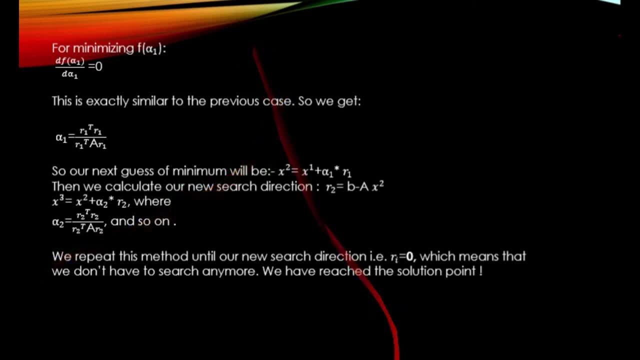 point. well, for minimization of F of alpha 1, finding the derivative of alpha 1 with respect to alpha 1 and equating with 0, you get: alpha 1 is equals to r1 transpose times r1 divided by r1. 1 transpose times a times r 1. so now our guess of minimum will be x. 2 is equals to alpha 1 plus. 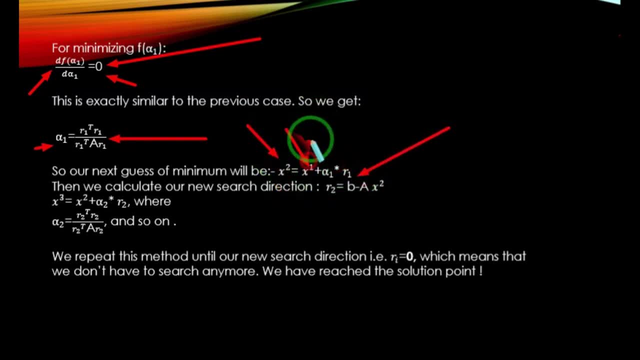 sorry. x 2 is equals to x 1 plus alpha 1 times r 1. then we calculate our new search direction, r 2, which is given by b minus a times x 2. again we find x 3 using x 2 plus alpha 2 times r 2, where 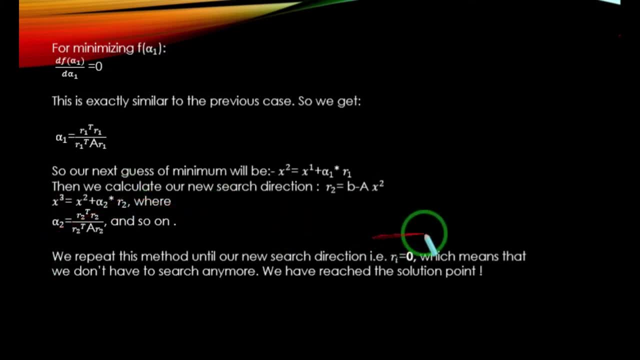 alpha 2 is given by r 2, transpose times r 2 divided by r 2. transpose times a times r 2, and so on, guys. oh my god, i'm tired. well, we repeat this method until our new search direction, that is: r i is equal to x 2 plus alpha 2 times r 2, and so on. 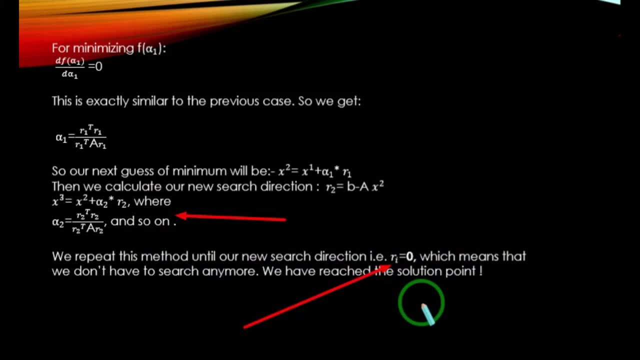 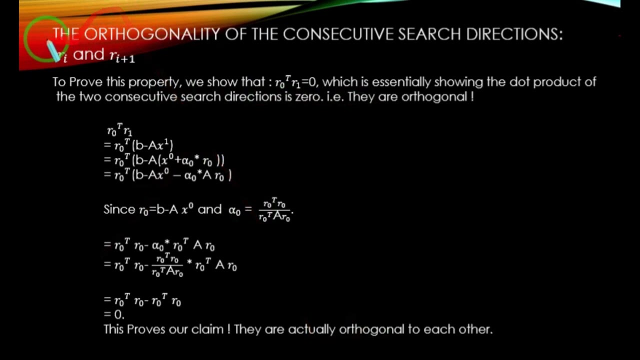 equals to 0, which means that we do not have to search anymore. well, we have reached the solution. now the next thing to know in this concept is the orthogonality of the consecutive search directions, which basically means that suppose you have r1 as the initial search. 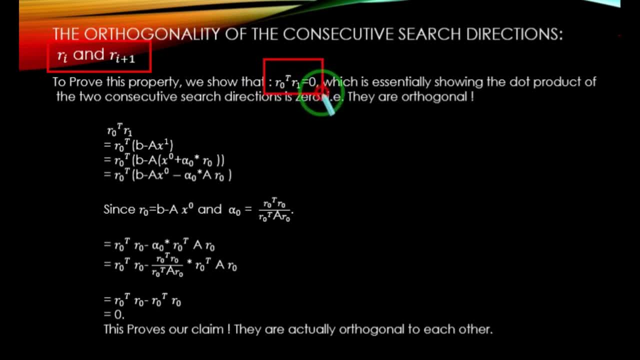 direction and r2 as the second search direction, then they are supposed to be perpendicular according to zero. and now, in this case, if we laught and run the previous lecture, this was already revealed right and now. if we laught the previous lecture and then we laught and run the recent lecture and then and 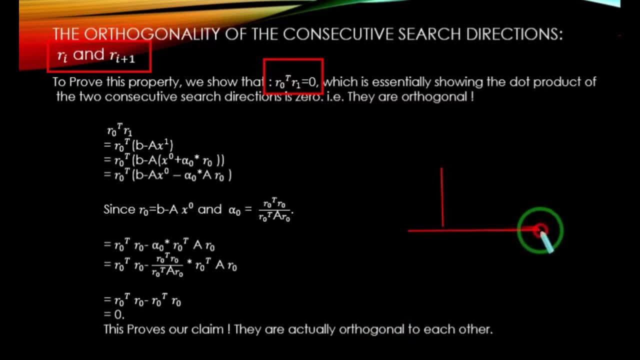 they are supposed to be perpendicular according to zero, and here r1 would be 1. transpose times a times x, 2 and this concept. well, let's prove it now. to prove this property, we shall show that x naught transpose times x1 is equals to 0, which is essentially showing that the dot product of the two 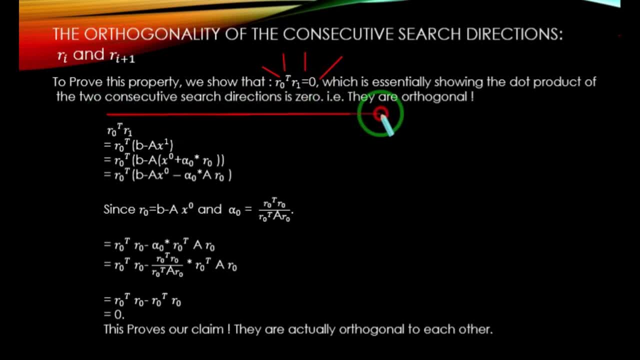 consecutive search directions is zero, that is, they are orthogonal. well, x naught transpose, sorry r naught. transpose times r1 is equals to r naught. transpose times b minus a x1, which is equals to r naught. transpose times b minus a x naught plus alpha: naught times r naught, and so. 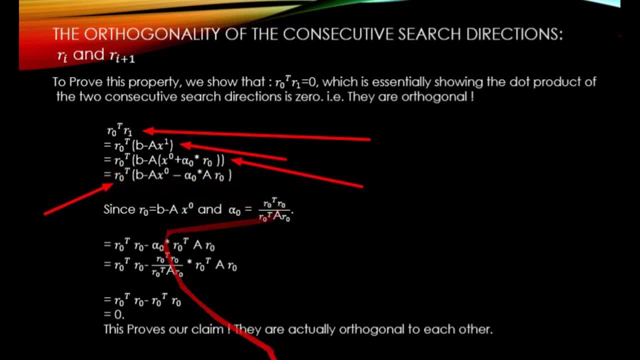 on guys, so on, so on, so on. well, since r naught is equals to b minus a times x naught, and alpha naught is equals to r naught, transpose times r naught divided by r naught. transpose times a times r naught. substituting these values, you finally come to this point: zero. yes, the dot product has found to be. 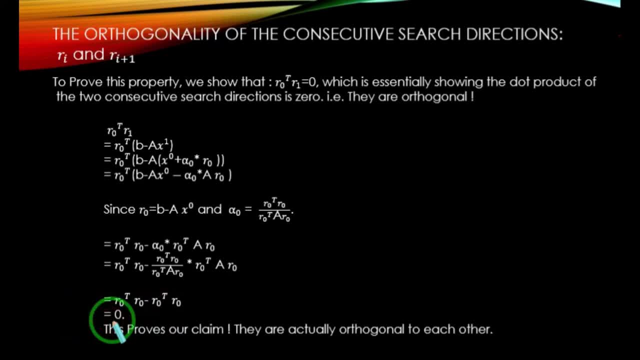 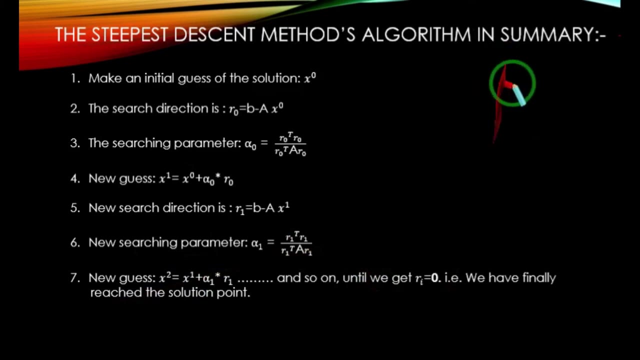 zero. well, this proves our claim that they are actually orthogonal to each other. well, that is all, guys. that is all. well. if you simply want to know the algorithm with the steepest decent method, here is the list. firstly, make sure that an initial guess of the solution is taken, which is x, naught. secondly, such detection is taken to be r naught. 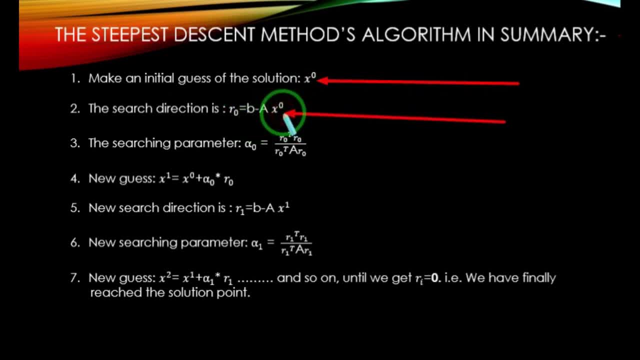 which is equals to b minus a times x naught. thirdly, the surging parameter alpha is equals to r naught transpose times r, naught divided by r. naught transpose times a times r. in fourth point, fourth step, now new guess is given by x1, which is equals to the previously. 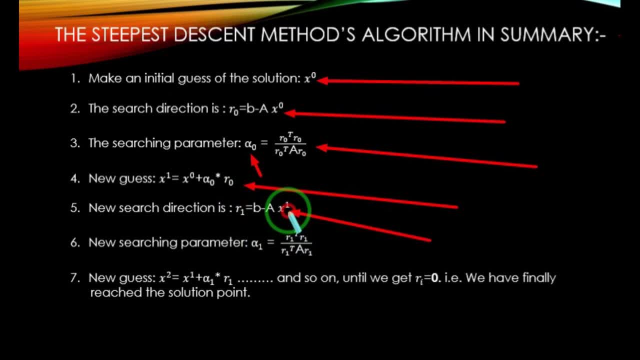 used x naught plus alpha naught times r naught. new search direction: is given by r1, which is equals to b minus a times x1. and sixth step: you find the new searching parameter, alpha 1, which is given by r1: transpose times r1 divided by r1. transpose times a times r1. now the new guess. 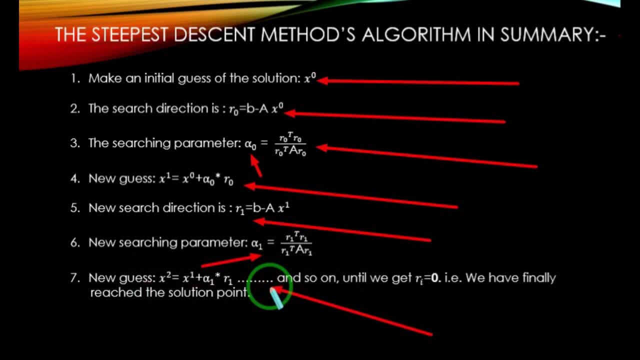 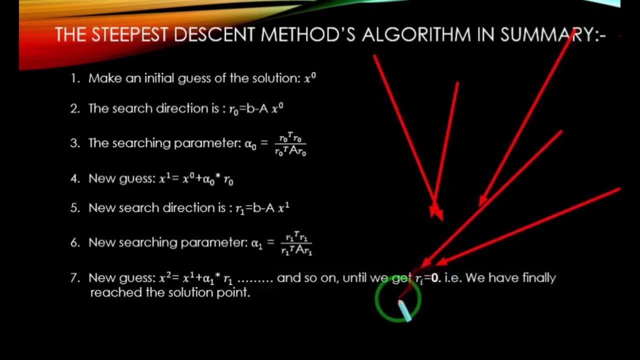 again is: x2, is equals to x1, plus alpha 1 times r1, and so on, and so on, and so on, until you get r i r something equal to zero, yes, r something, and we finally reach the solution, guys, we finally reach the solution point. 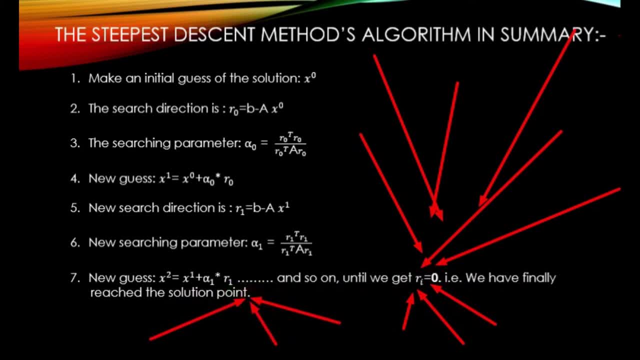 and it's over finally. oh my god, this was hard. thank you, guys for watching this video. do like, comment and subscribe and please, please, please, share this video, because i'm tired you.